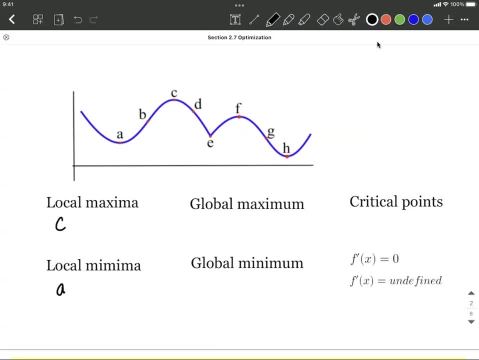 C looks to be a highest point, so it goes as a maximum. It also appears to be the very, very highest point on the entire graph, so that would be the global maximum. All right, D is kind of in the middle there, so it's not going to be a maximum or a minimum. E. 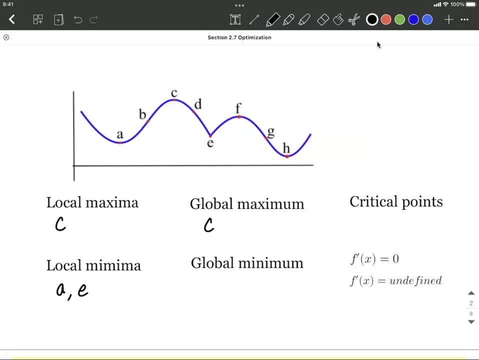 is going to be a minimum, or minima is another way to say that. And then let me see: F appears to be at the top of a hill, so it goes as a maxima, but not the very highest point, so it's not the global maximum. G is kind of in the middle, not the highest or the lowest. 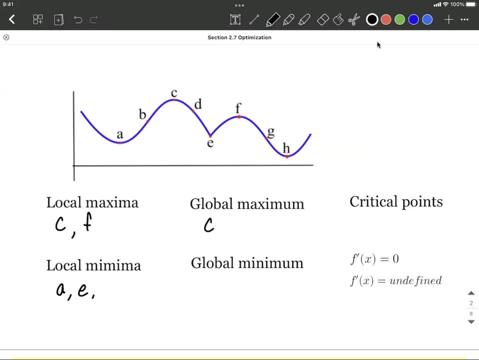 in that section, And H appears to be a lowest point, so it's going to go as a minima. Now it also appears to be the very lowest point on the entire graph, so I'm going to go ahead and classify it as the global minimum. Now, they didn't point out these endpoints on the 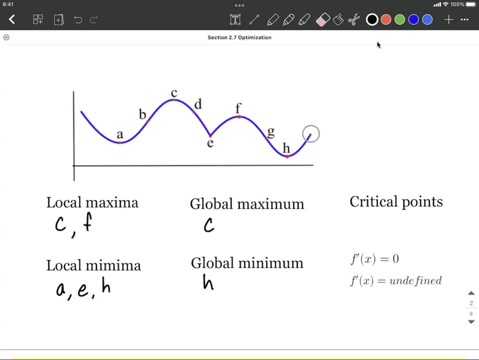 graph. Typically, if we have a nice filled-in circle at the end, like we appear to, we're going to go, that would also get classified. This one would be a maximum, and on the left-hand side would also be a maximum. They don't appear to be the very highest point on the entire graph, so it would 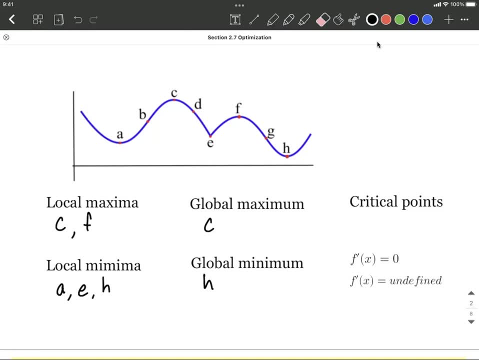 only be a local or relative maximum. All right, now critical points. Critical points occur whenever the first derivative is either equal to zero or would be undefined. So that means the slope of the tangent line would be horizontal if the first derivative equals zero. That's going to happen. 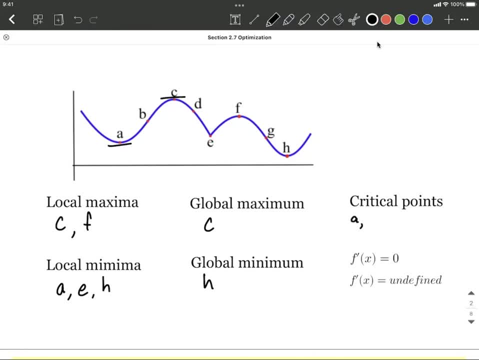 here at C, and now it doesn't happen at B. right B is going to be. you know about a slope of one, so the first derivative would equal one at B, D, no, E is kind of unique on this. Now E would 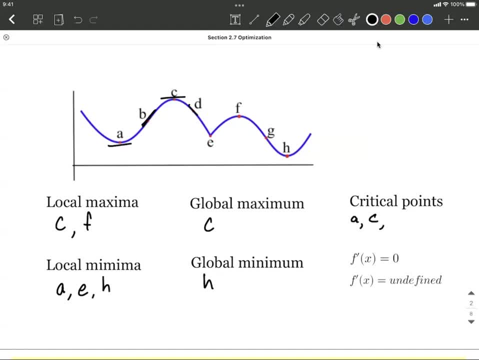 actually be undefined, so that actually goes as a critical point. All right, undefined meaning like a vertical line would be the tangent line If we were to try to draw one in. we typically do not. when we have a sharp corner, though, is what. 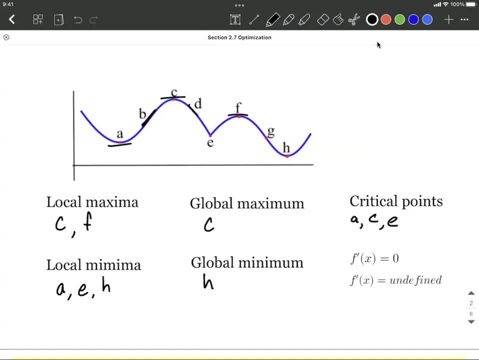 you can be looking for on a graph. All right, F has a horizontal tangent line, so it gets classified as a critical point, and H would also have a horizontal tangent line, which goes as a critical point as well. Now, one takeaway you may have is taking a look at all these critical points.